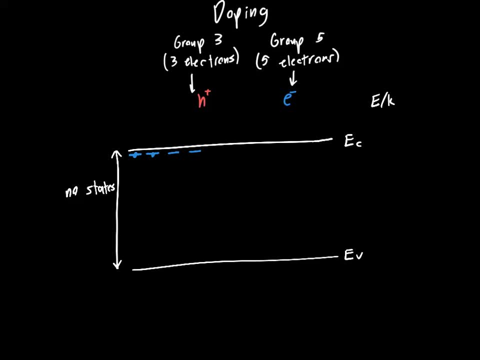 that initially contain an electron. so we've got a bunch of states that each have an electron and here the electrons are just these little blue circles and so at temperature of zero degrees Kelvin these electrons- add the electron in a actually can't move up to the conduction band, So in these states they can't actually conduct. 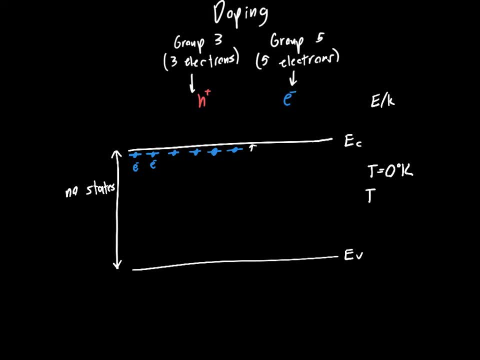 electricity And as you start to raise the temperature- so say to T equals one degree Kelvin- maybe, maybe some of these electrons can hop up into the conduction band and start conducting electricity, but not too many, As you start to raise the temperature higher and higher. 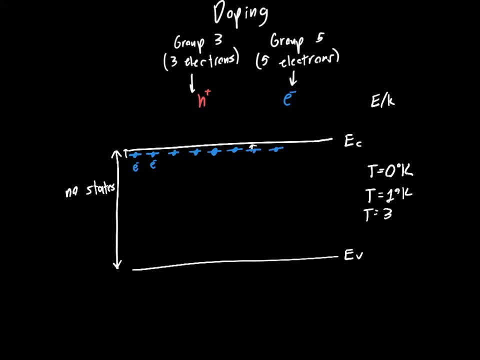 and by the time you get to room temperature, T equals 300 degrees Kelvin, then most, if not all of the- well, most- of these electrons have jumped into the conduction band because they have enough just thermal energy from random movement to jump up into the conduction. 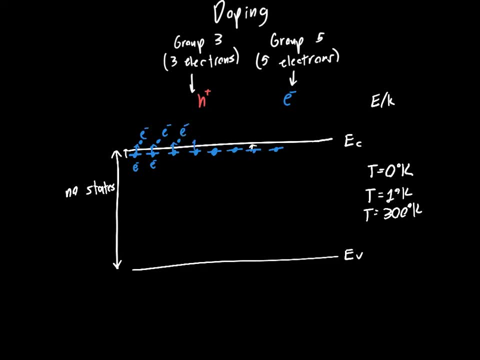 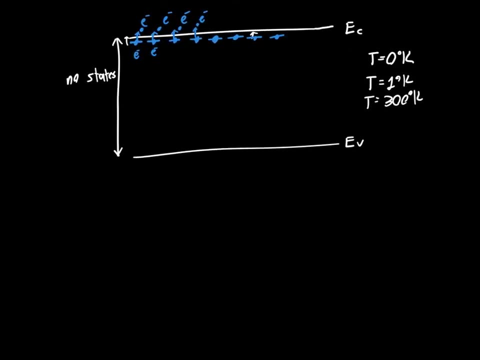 band, And so these electrons are now available to conduct electricity. And similarly, if we dope the semiconductor with rather than with a type four, what type five? semiconductor with a group five? semiconductor with a group three semiconductor? we've got our conduction band and our valence band. We've got a bunch of 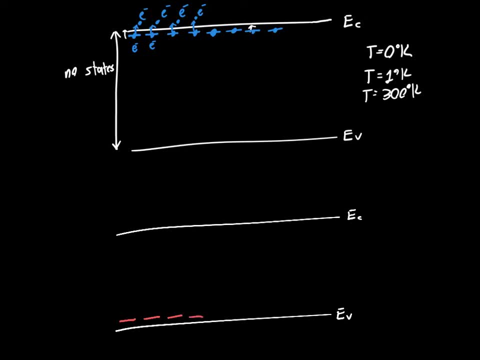 empty states here, except they're empty in the sense that they have an extra. they have an extra hole, So they- you can think of them as being devoid of electrons or as containing a bunch of holes, And so at T equals zero Kelvin, these holes have no energy, they have no thermal. 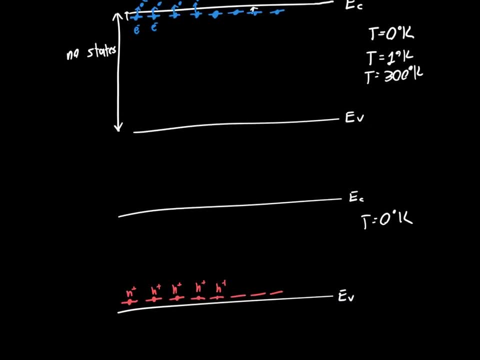 energy They cannot move. And then, as we start to raise the temperature a little bit, a couple of them are going to start to be able to escape. and then, as we get to room temperature, Almost all of them have enough energy to escape into the valence band and start conducting. 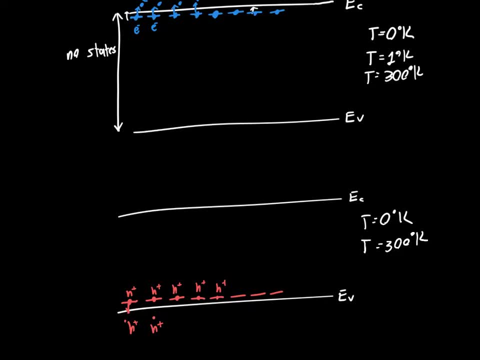 electricity And just to give you a sense of scale, these, uh what are called ionization energies, are typically on the order of like 40 milli EV, which is really tiny Um. the KT, the thermal energy, is about 26 MEV Um, so at room temperature on average, uh, there's, there's plenty of energy. 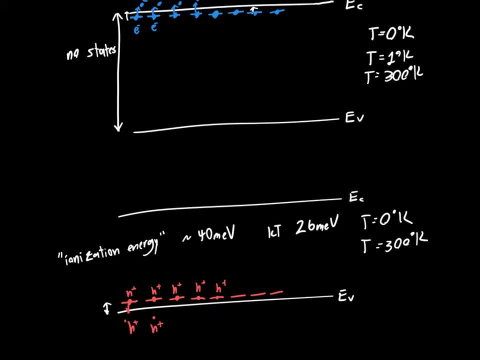 for these, for these donors to be ionized, And the number of ionized donors uh doesn't just depend on the ratio of KT and the ionization energy. It depends, uh, on the quantum mechanics behind it, So on the Fermi direct distribution for these uh, for these donors. but we're not. 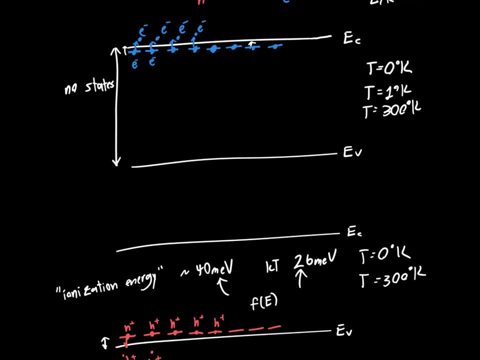 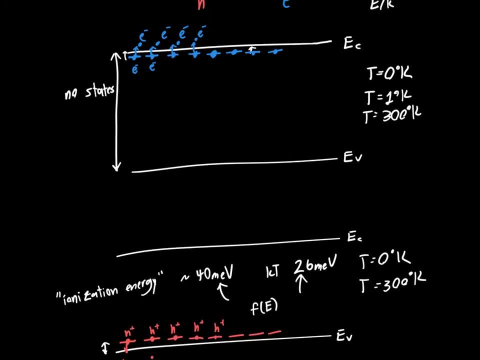 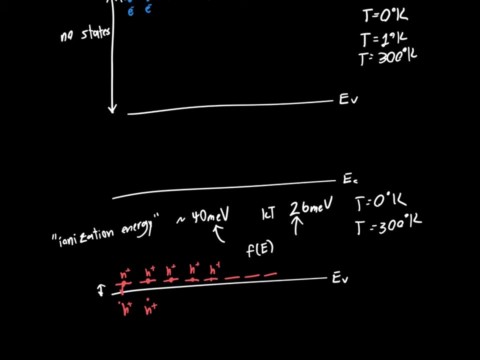 we're not going to analyze that uh, that here. So if we look at this from a band diagram perspective, we're introducing either additional electrons with their additional accompanying states and additional holes with their accompanying states, And you might say, well, once the electron leaves, uh say this is now. 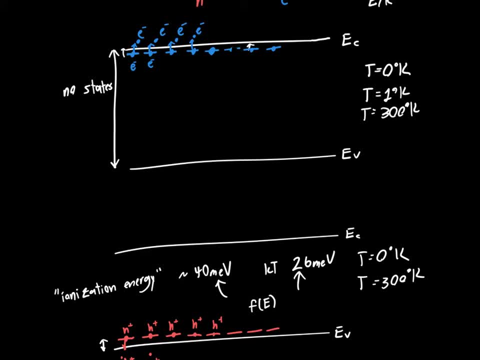 up here say this is an empty state. So we've got our our empty state here. Uh, can an electron down here in the valence band jump up into the valence band? So we've got our our empty state here. Uh, can an electron down here in the valence band jump up into the valence band? 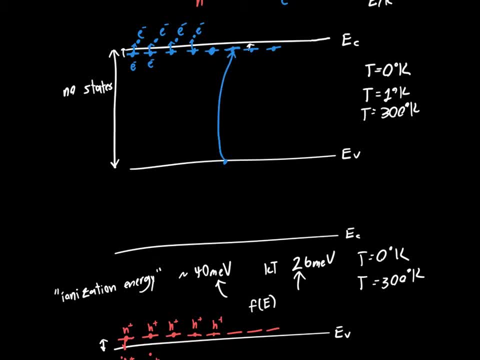 So we've got our empty state here. Uh, can an electron down here in the valence band jump up into the valence band? Uh, and then conduct electricity? Well, yeah, yeah, it can. uh, electrons can jump into these. 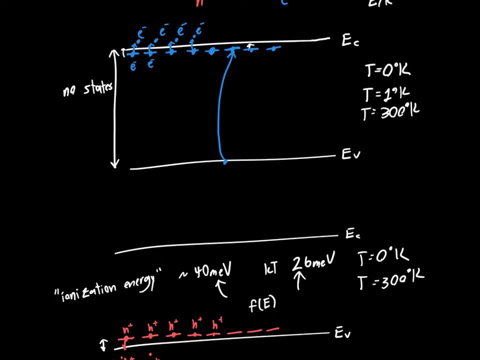 states, just as they jump into the conduction band, And then it can just make the little hop here, uh, into the conduction band and it can start conducting electricity. So, yes, those states are free. Uh, they, they are, except accessible to the electrons. Um and same same with the holes Now. 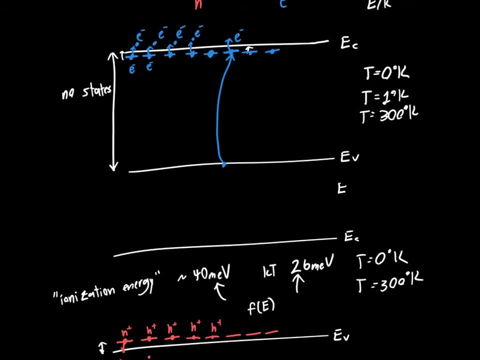 I've been uh sort of alluding to this Fermi energy in the equations that we've used, so in the Fermi direct distribution and now in the concentration equations for electrons and holes, and We haven't really talked much about the Fermi energy or how it's affected by doping or 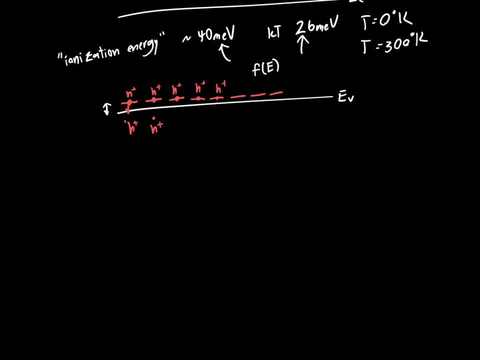 What it really, what it really means. Well, remember, last time we derived the equation that the Number of electrons is just equal to this constant out front, which is a function of temperature, at times e to the minus EC, minus EF Over KT, and so we would expect that the Fermi energy EF. 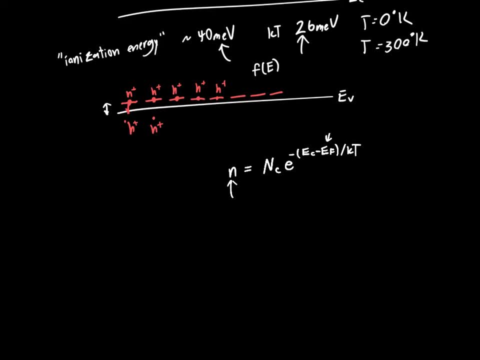 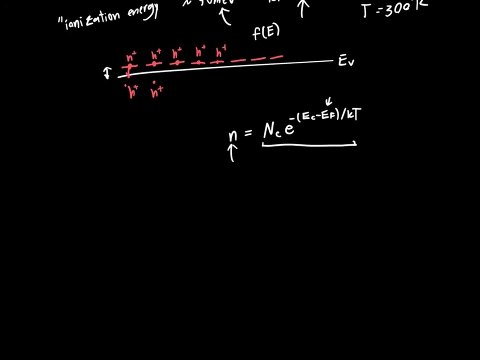 Depends on the electron concentration. so if we change the electron concentration through doping, Since this equation is always true- Then this side has to change. and since NC doesn't depend on anything to do with with doping, It's EF that has to change in this equation. so the Fermi energy gives us, and the Fermi level gives us, an indicator of 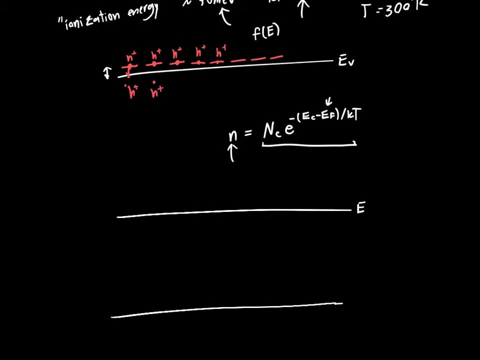 Which type a Semiconductor is. so, whether it's n-type or has an excess of electrons, or p-type, has an excess of holes. So if we have an n-type semiconductor, We've got a bunch of states up here and I'm assuming that they've donated their electrons now to the conduction band. 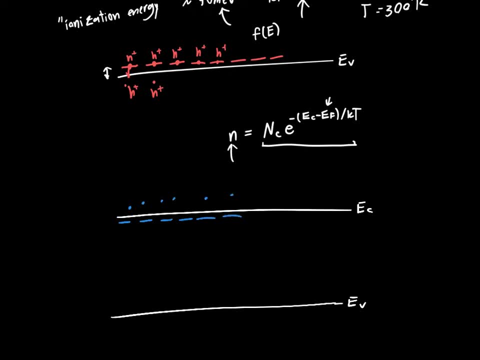 So we're at a nonzero temperature, Then we would expect the Fermi energy- Or you can think of it intuitively, like the Fermi energy is kind of dragged up By all of these extra states, or if you just want to derive it mathematically, you see that well. 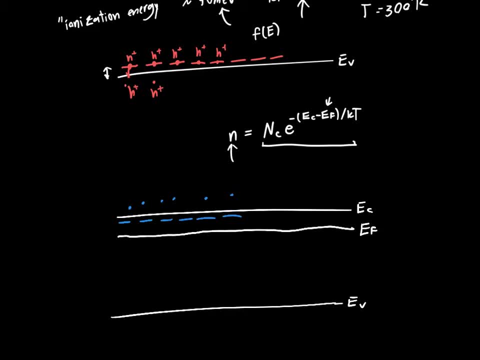 If n goes up, Then this whole term over here must go up or the Fermi energy Must go up, since it's a negative of a negative in an exponential. so these dopant states, these group five Donor- They're often called donor states Because the they're donating an electron- drag this Fermi energy up to the top of the 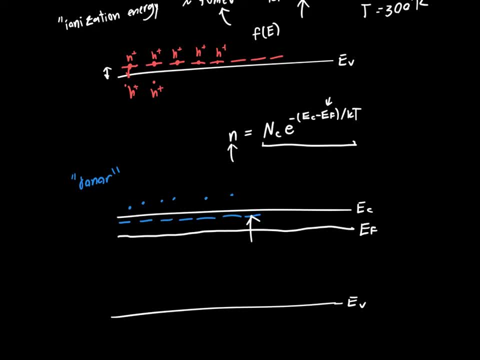 of the band diagram. So we're kind of starting to get a more complete band diagram and this is going to be really useful for analyzing the PM junction, analyzing MOSFETs. It's going to be an indispensable tool that we really need to get familiar with. 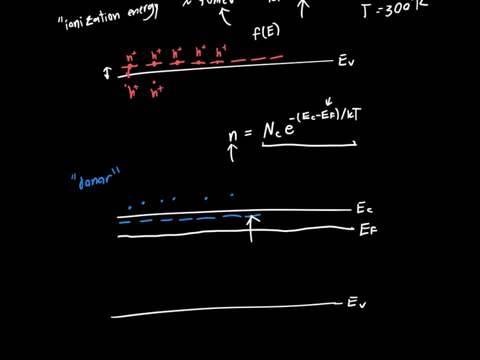 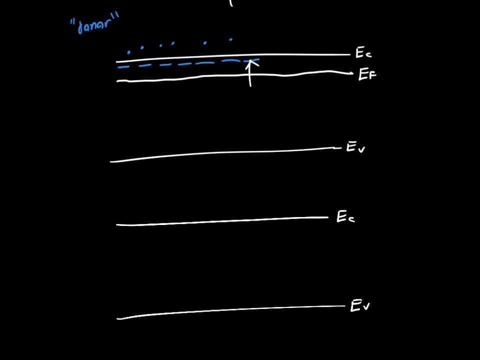 So, similarly, if we have a semiconductor that we choose to dope with a bunch of donor, or a bunch of acceptor states, as they're often called, with a bunch of acceptor atoms and, I'm assuming, a non-zero temperature, so we've got now a bunch of extra holes in the valence band which are available to conduct electricity. 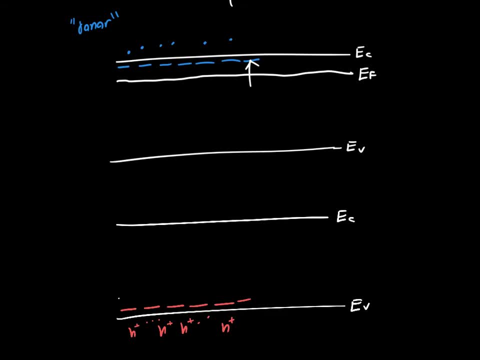 then the Fermi energy is going to be dragged down more towards the bottom. So this is a P-type semiconductor, this is an N-type semiconductor, and where the Fermi energy is located is really important and it's fairly easy to remember. if you just remember that, well, a P-type semiconductor, the Fermi energy will be dragged towards the valence band because all these holes are kind of dragging the Fermi energy. 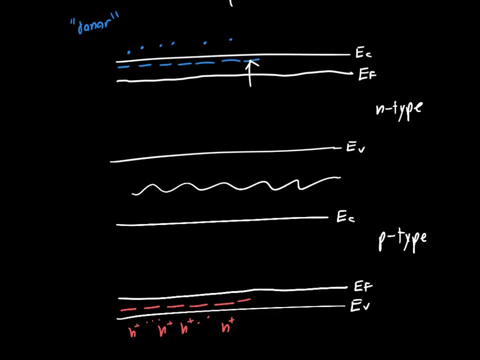 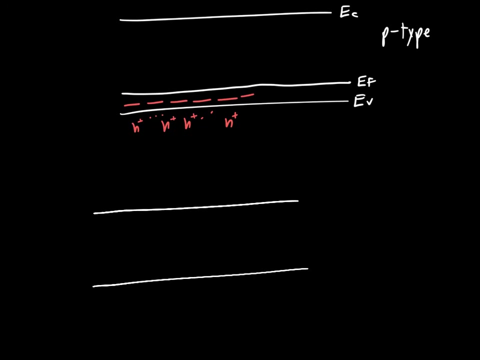 Now that's not a physical explanation but it sort of helps. it's an intuitive way of remembering. Similarly, these electrons are dragging the Fermi energy up towards the conduction band. so we see that this Fermi energy, EF, kind of gives an indicator of the type of the silicon. and so we'd expect that at if we didn't add any dopant and we had our conduction band and our valence band, we'd expect the Fermi energy to be somewhere in the middle. 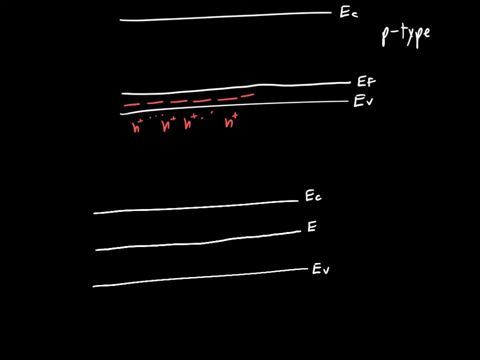 We'd expect the Fermi energy to be like somewhere here And this is often called EFI, EFI or the intrinsic Fermi level. so the intrinsic refers to the semiconductor, the undoped semiconductor, it's just intrinsic This, so the Fermi level is at a location EFI, and a lot of times and in most of the future band diagrams I draw, I'll kind of draw this as a dotted line just to serve as a reference for whether, for basically where the midpoint is. 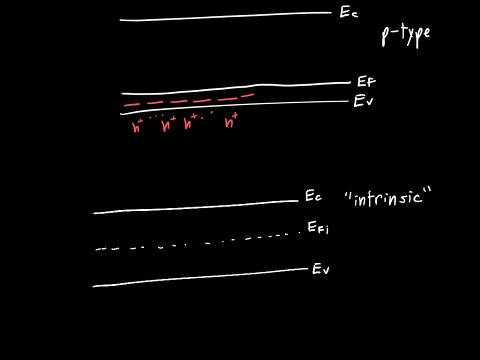 And the intrinsic Fermi. The Fermi concentration isn't exactly or the Fermi level isn't exactly at the midpoint, but it's pretty close and I'll go over in a future video where exactly it is. So this intrinsic Fermi level allows us to easily visualize. well, if I've got a Fermi energy near the top above the intrinsic Fermi level, it's definitely an n-type semiconductor.